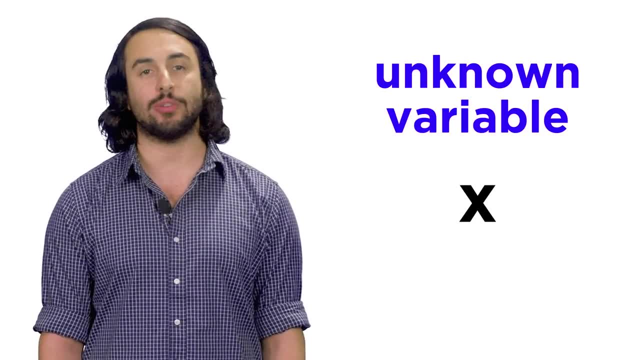 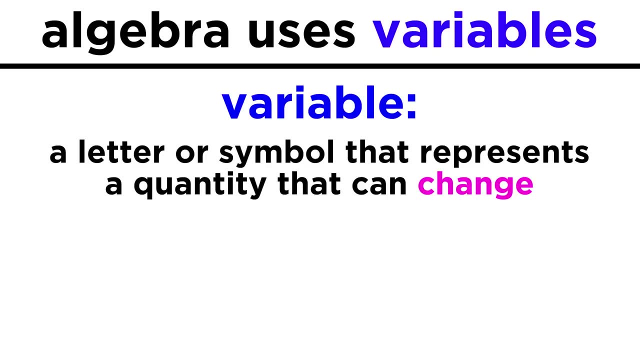 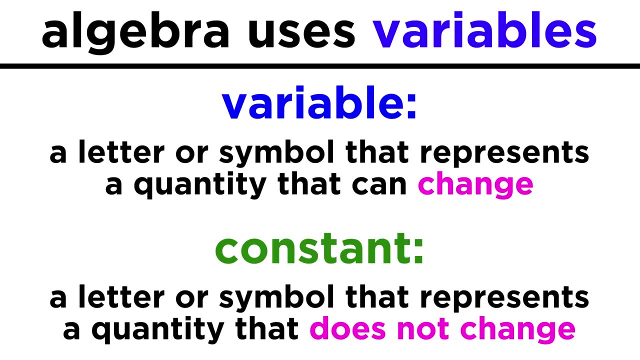 equations. Let's start out by discussing that algebraic essential: the unknown variable. First of all, what is a variable? In math, a variable is a letter or symbol that represents a quantity that can change. This is different from a constant, which is a letter or symbol that can change. 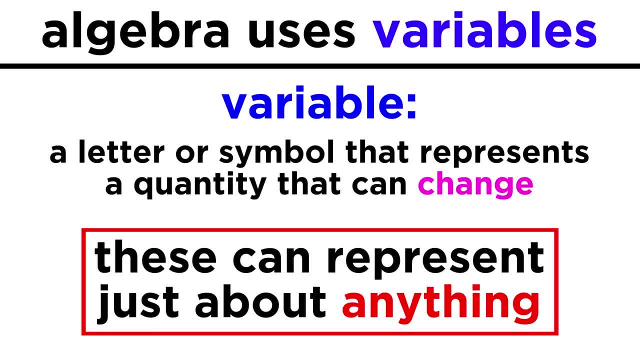 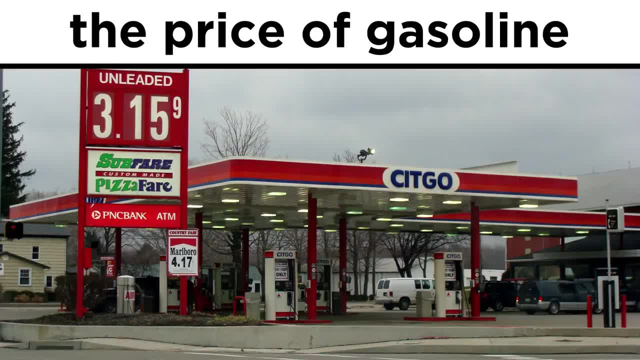 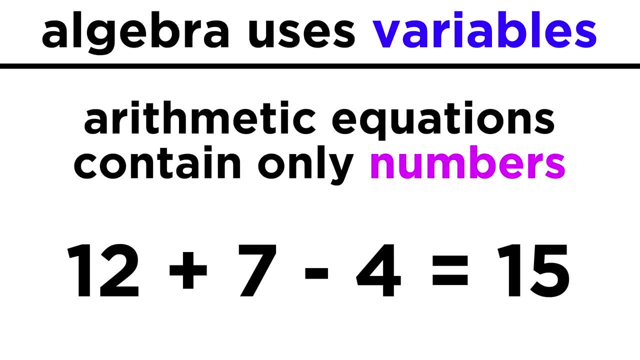 A variable can be just about anything: The inches of rain in your town in a particular month, the price of gasoline, the speed of a plane, whatever it is that you want to do math with- Whereas with arithmetic, our equations simply contain numbers and arithmetic operations. 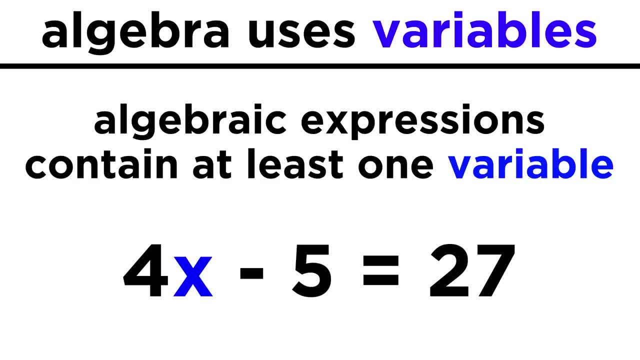 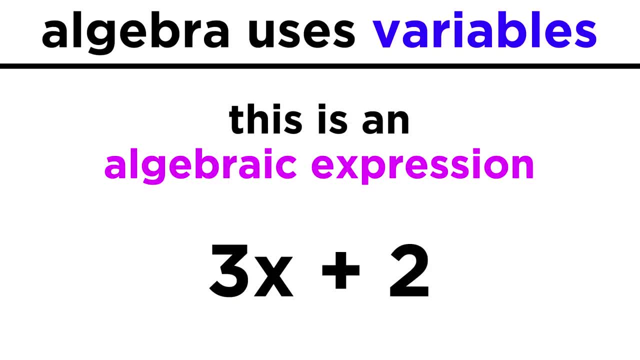 an algebraic expression will always include one or more variables, as well as some numbers. So what is a variable? A variable is a number. It contains some numbers and operations. For example, three X plus two is an algebraic expression. We can evaluate this expression for any value of X that we choose. 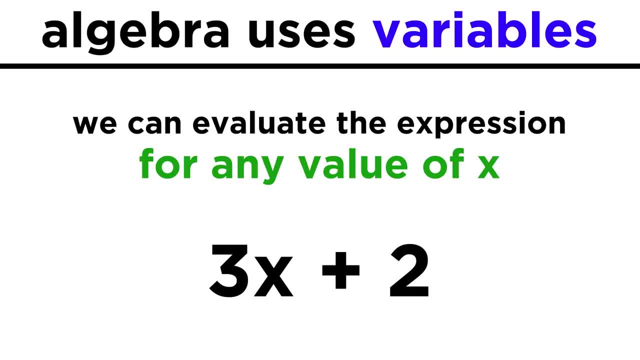 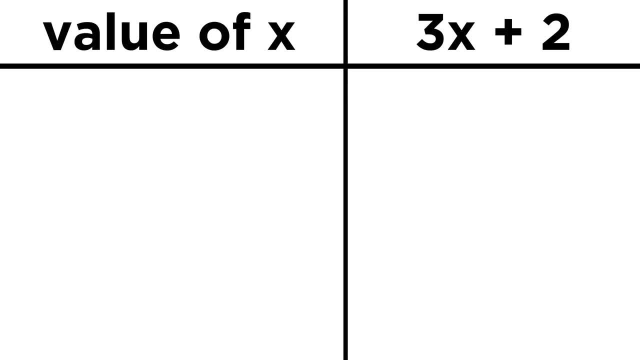 We simply plug the value into the expression, understanding that we can now represent the multiplication of two numbers by simply placing them next to each other. We could make a table as we do this. When X is one, we replace the X with a one. 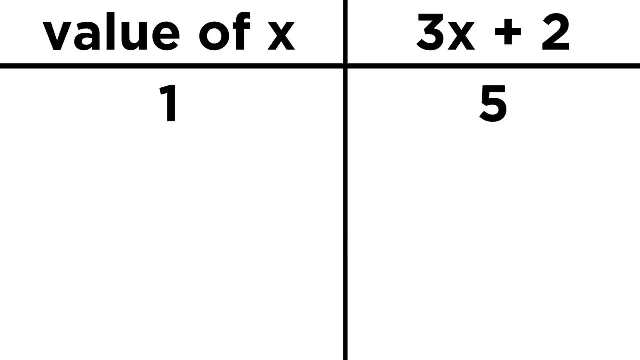 Three times one is three Plus two is five. so when X is one, this expression is equal to five. When X is two, we get six plus two or eight. When X is three, we get nine plus two or eleven, and so forth. 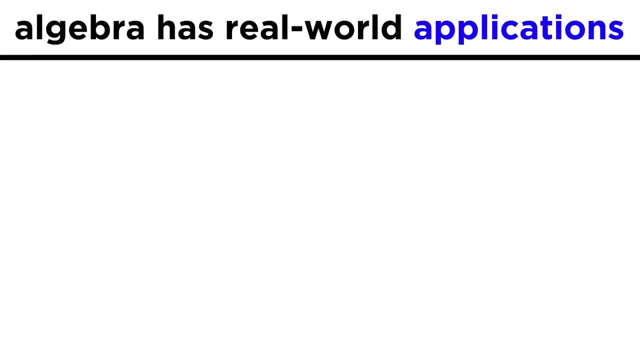 This is useful because we can use algebraic equations to model real world situations and make meaningful statements about them. Instead of just using arithmetic to say that five cheeseburgers at three dollars each will cost a total of fifteen dollars, we can set up an algebraic relationship that allows us to do a wide 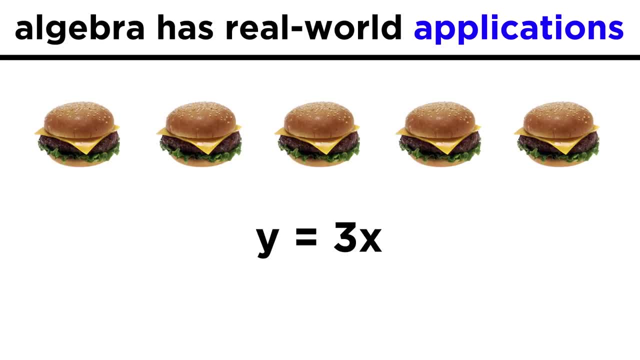 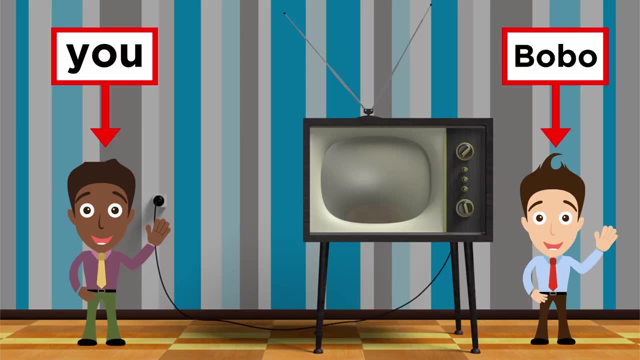 variety of calculations that are pertinent to this situation, like how: Y, the total cost is equal to three times X the number of cheeseburgers. The trick is just knowing how to set up the equation. Let's say that you love to watch TV, but not as much as your friend Bobo. 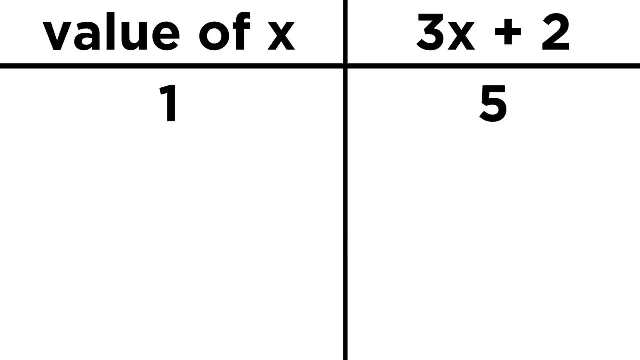 Three times one is three Plus two is five. so when X is one, this expression is equal to five. When X is two, we get six plus two or eight. When X is three, we get nine plus two or eleven, and so forth. 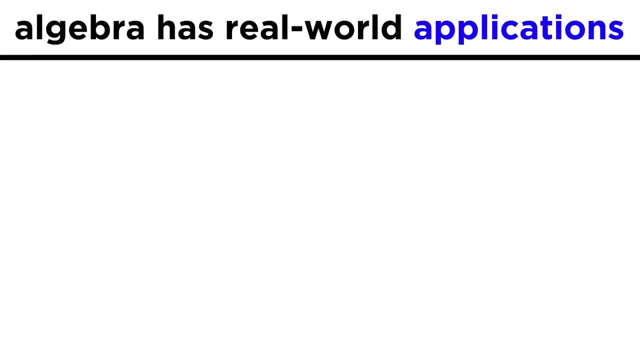 This is useful because we can use algebraic equations to model real world situations and make meaningful statements about them. Instead of just using arithmetic to say that five cheeseburgers at three dollars each will cost a total of fifteen dollars, we can set up an algebraic relationship that allows us to do a wide 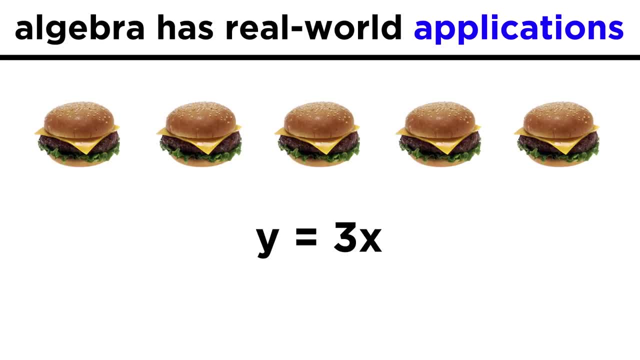 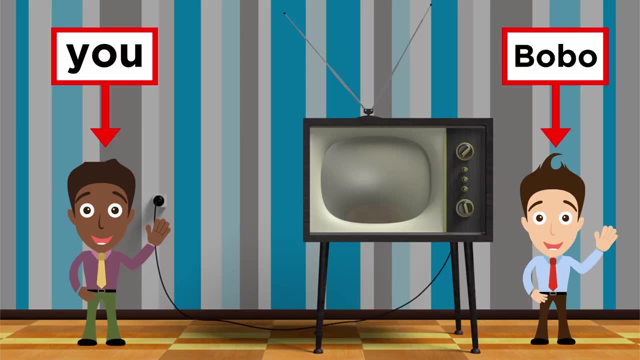 variety of calculations that are pertinent to this situation, like how: Y, the total cost is equal to three times X the number of cheeseburgers. The trick is just knowing how to set up the equation. Let's say that you love to watch TV, but not as much as your friend Bobo. 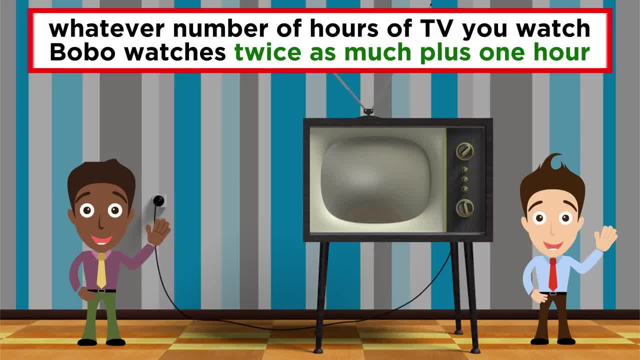 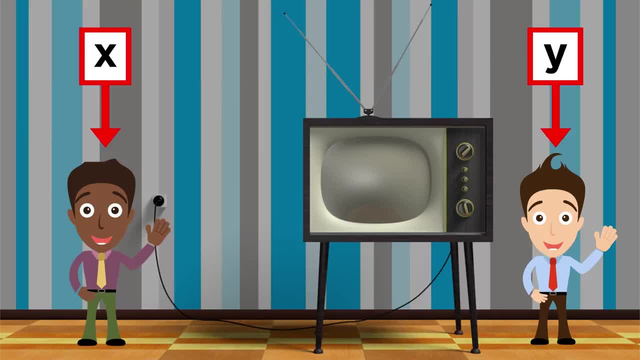 However many hours of TV you watch in a day, Bobo watches TV. He's not a big fan of TV, He likes to watch TV. Bobo watches twice as much plus an additional hour. Well, if you watch X hours of TV and Bobo watches Y hours of TV, we can relate X and 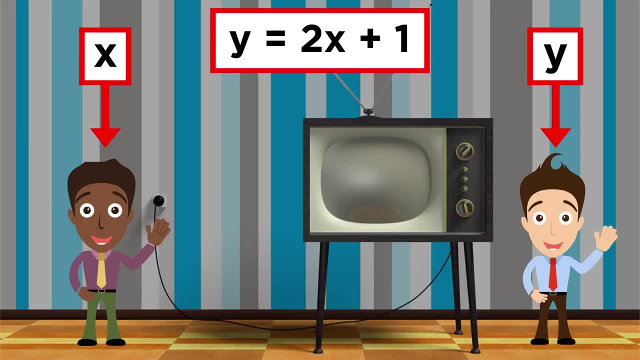 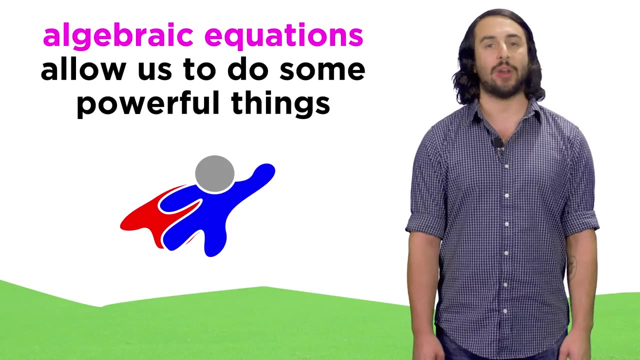 Y with an equation- just like we did for the burgers- where Y equals two X plus one. Whatever you watch which is represented by X, we double it and add one to get Y, the amount Bobo watches. While that was a pretty trivial example, these kinds of algebraic relationships allow us. 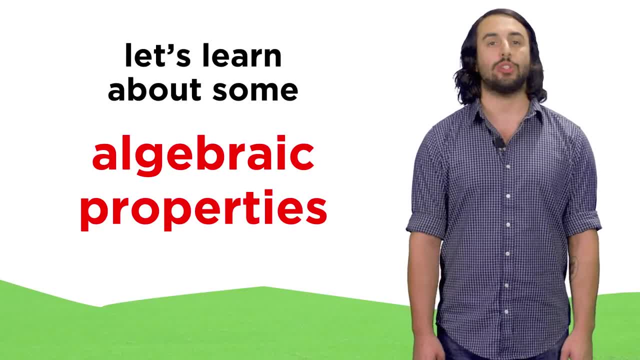 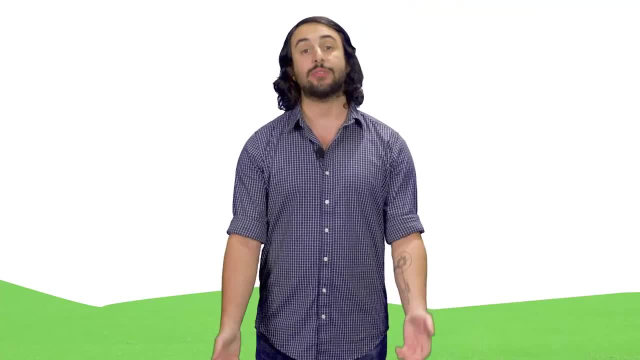 to do some pretty powerful calculations Before we start doing lots of algebra. there's a bit more to learn about algebraic properties, so let's move forward now. Thanks for watching, guys. Subscribe to my channel for more tutorials. support me on Patreon so I can keep making. 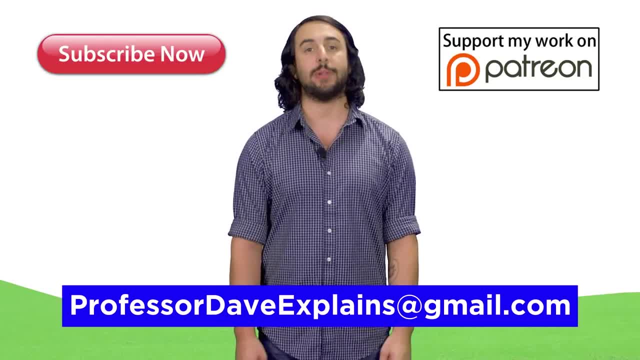 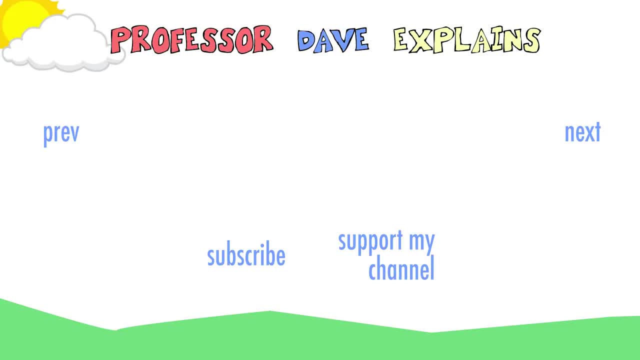 content and, as always, feel free to email me professordaveexplains at gmail dot com. I'll see you in the next video. bye.